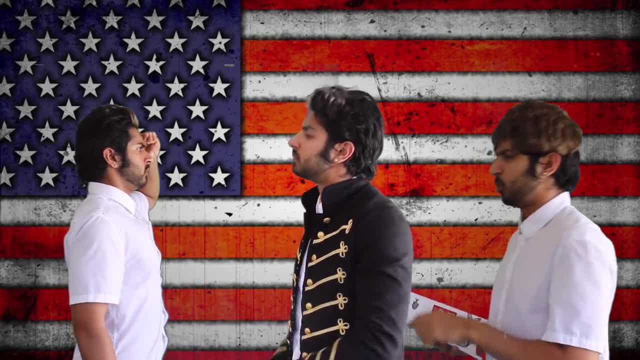 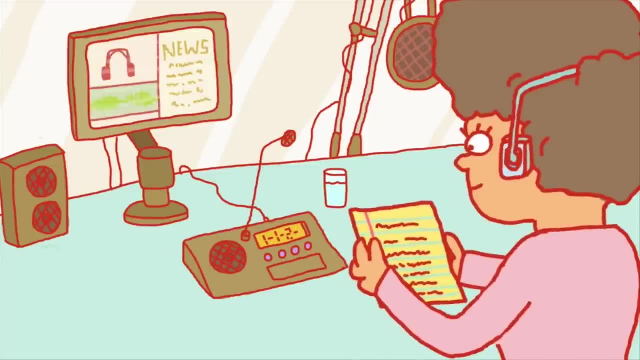 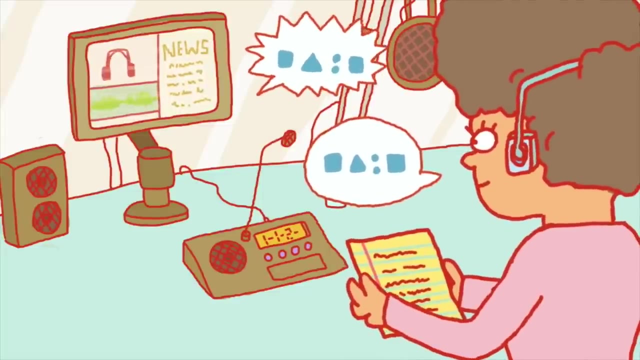 government learned of their translation effort. they were inspired to try it themselves post-war, specifically because they needed a way to keep up with Russian scientific publications. The first public demo of a machine translation system translated 250 words between Russian and English in 1954. It was dictionary based, so it would attempt to match the 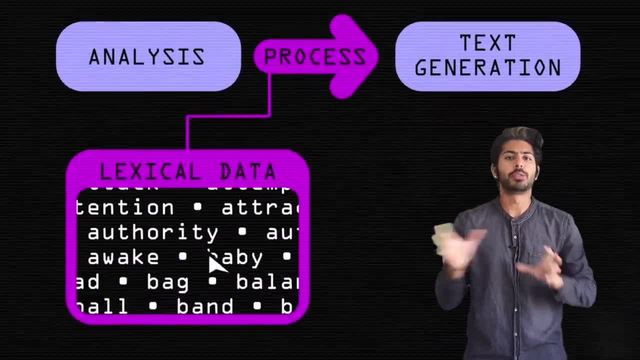 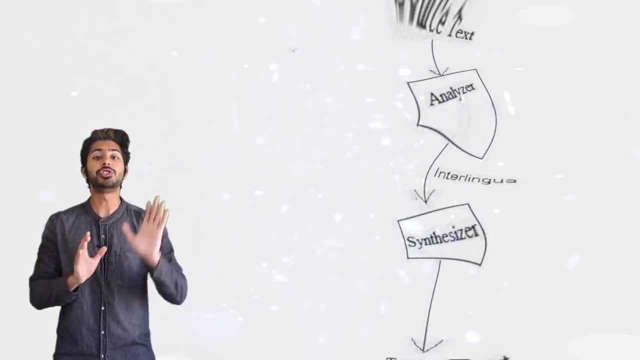 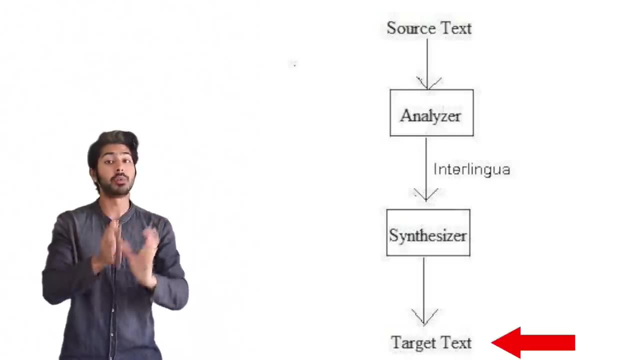 source language to the target language word for word. The results were poor since it didn't capture syntactic structure. The second generation of systems used intralingua. That means they changed a source language to a special intermediary language with specific rules encoded into it, then from that generated the target language. This proved to be more efficient, but this 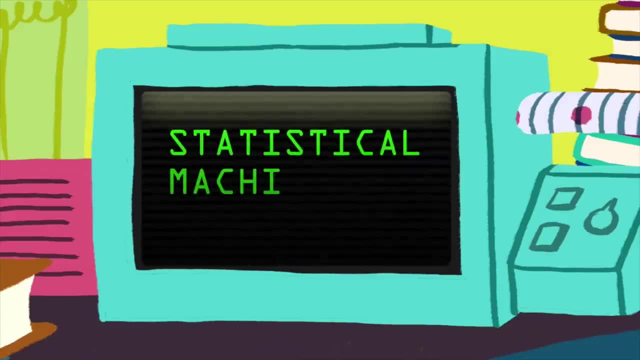 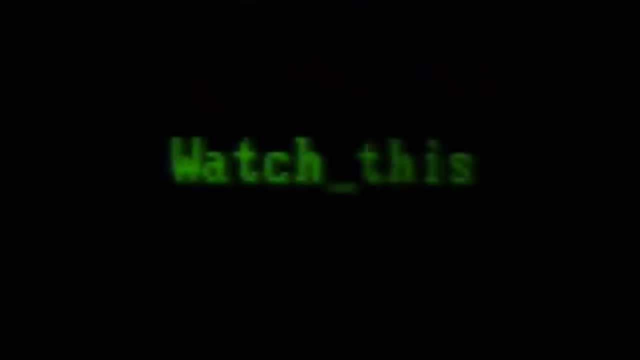 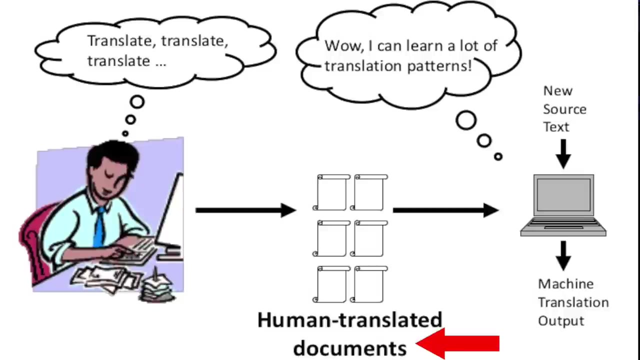 approach was soon overshadowed by the rise of statistical translation in the early 90s, primarily from engineers at IBM Innovation, at IBM watch. this A popular approach was to break the source text down into segments, then compare them to an aligned bilingual corpus, using statistical evidence and probabilities to choose the most. 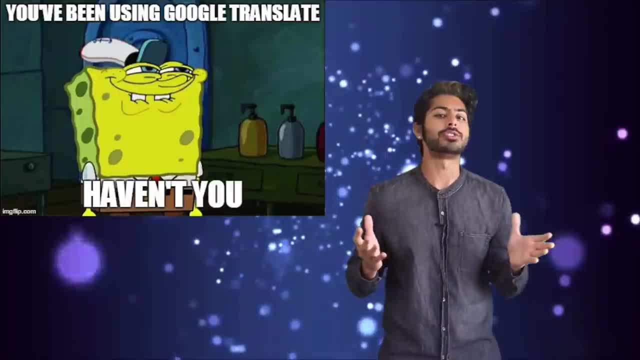 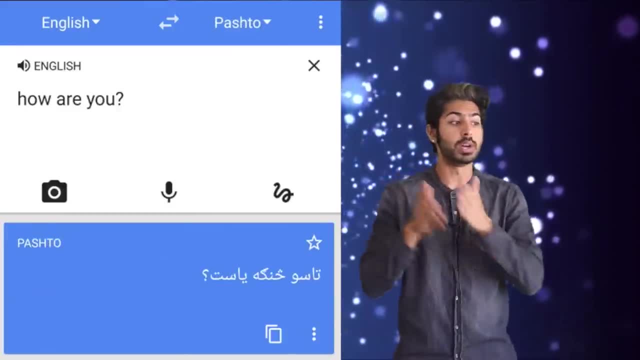 likely translation. Nowadays, the most used statistical translation system in the world is Google Translate, and with good reason. Google uses deep learning to translate from a given language to another, with state of the art results. So how do they do this? Let's recreate their results in TensorFlow to find out. 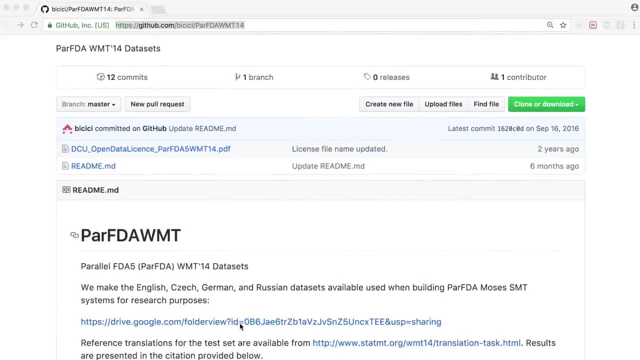 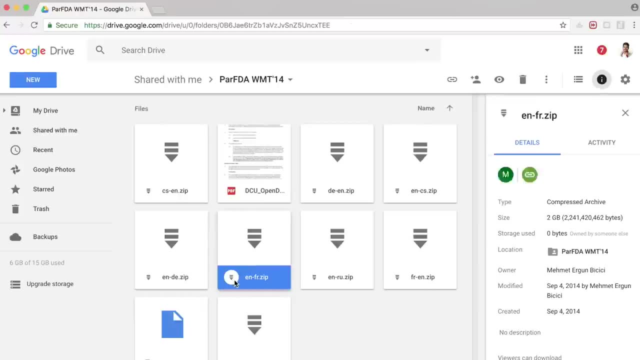 The dataset we'll be using to train our language translation model is a corpus of transcribed TED Talks. It's got both the English version and the French version, and our goal will be to create a model that can translate from one to the other after training. 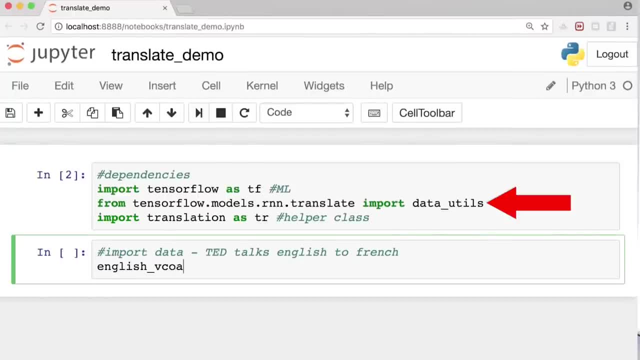 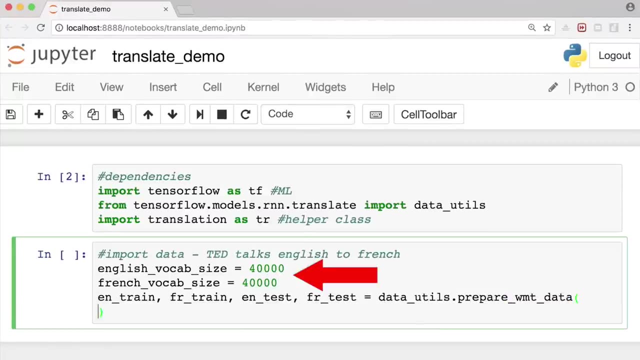 We'll be using TensorFlow's built-in data utils class to help us pre-process our dataset, and we'll start by defining our vocab size, which is the number of words we want to train on from our dataset. We'll set it to 40k for each, which is a small portion of the data. 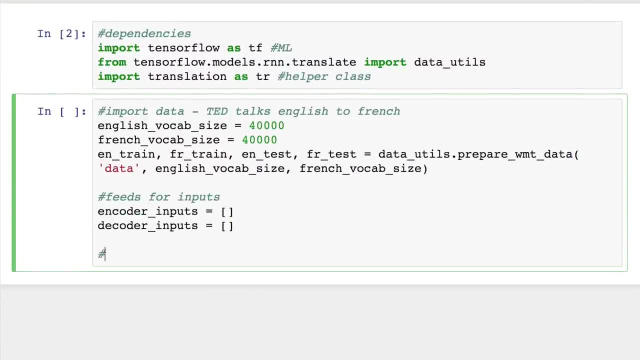 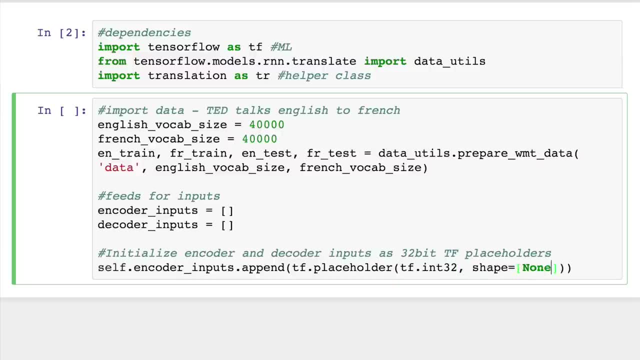 Then we'll use the data utils class to read the data from the data directory, giving it our desired vocab size, and it will return the formatted and tokenized words in both languages. We'll then initialize TensorFlow placeholders for our encoder and decoder inputs. 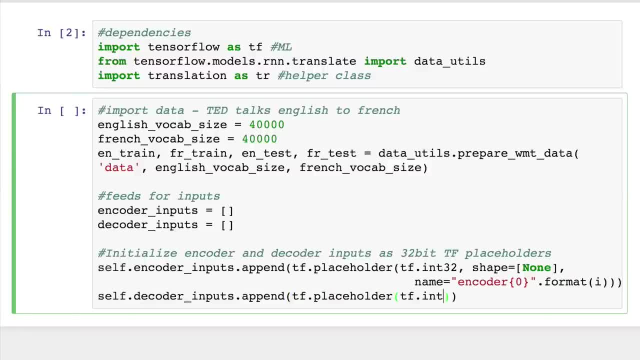 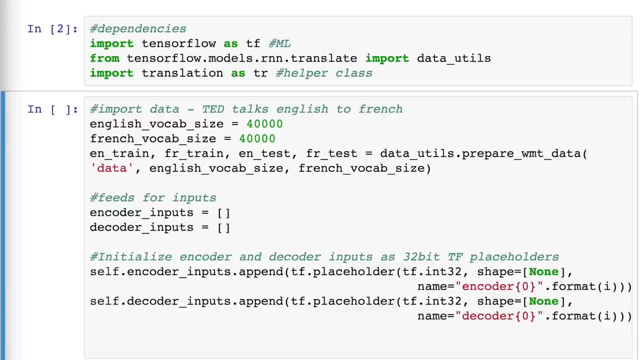 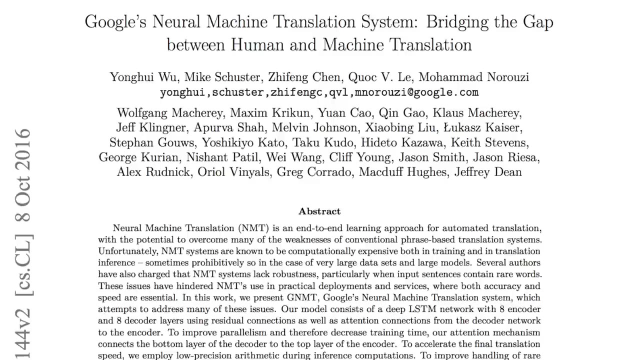 Both will be integer tensors that represent discrete values. They will be embedded into a dense representation. later We'll feed our vocabulary words to the encoder and the encoded representation that's learned to the decoder. Now we can build our model. Google published a paper more recently discussing a system they integrated into their translation. 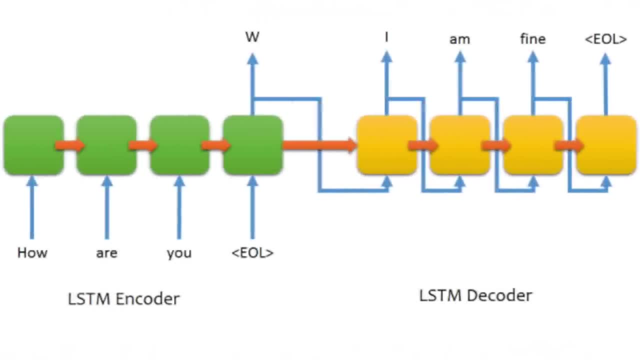 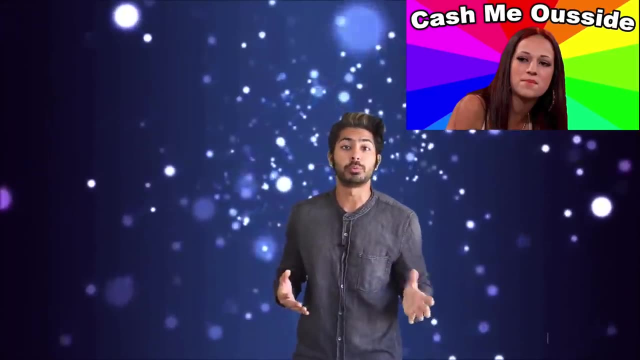 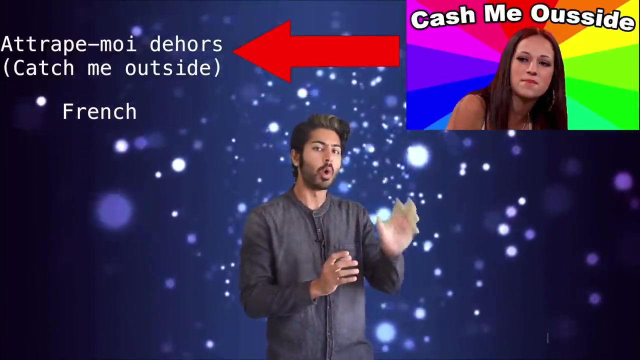 service called Neural Machine Translation. It's an encoder-decoder model inspired by similar work from other papers on topics like text summarization. So whereas before Google Translate would translate from language A to English to language B, with this new NMT architecture it can translate directly from one language to the. 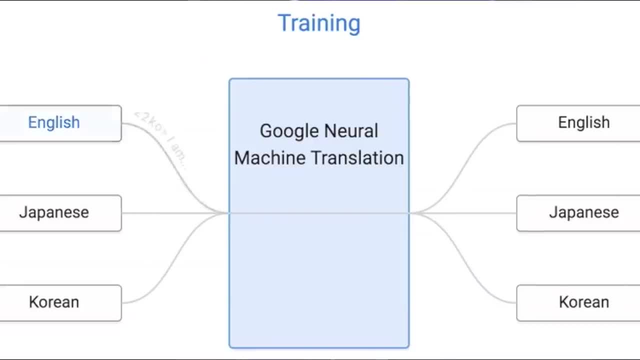 other. It doesn't memorize phrase-to-phrase translations. Instead, it encodes the semantics of the language So we can build our model. This encoding is generalized, so it can even translate between a language pair like Japanese and Korean that it hasn't explicitly seen before. 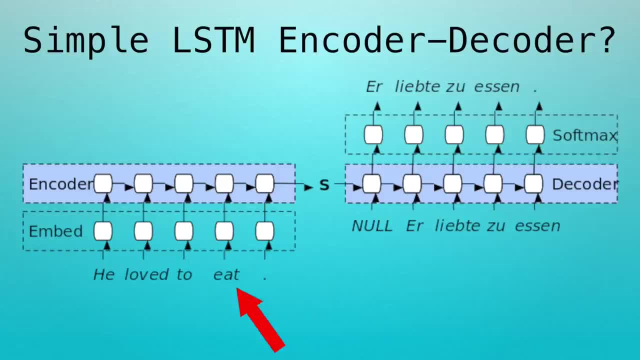 So I guess we can use an LSTM recurrent network to encode a sentence in language A. The RNN spits out a hidden state, S, which represents the vectorized contents of the sentence. We can then feed S to the decoder, which will generate the translated sentence in language. 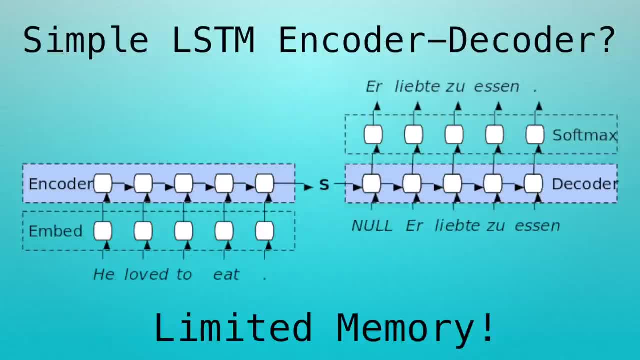 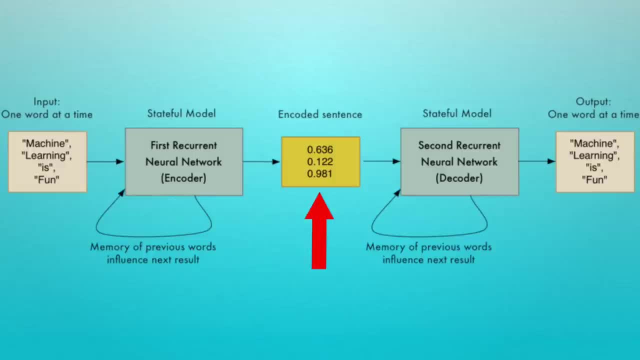 B, word by word, Sounds easy enough, right Wrong. There's a drawback to this architecture: It has limited memory. That hidden state S of the LSTM is where we're trying to cram the whole sentence we want to translate. S is usually only a few hundred floating point numbers long. 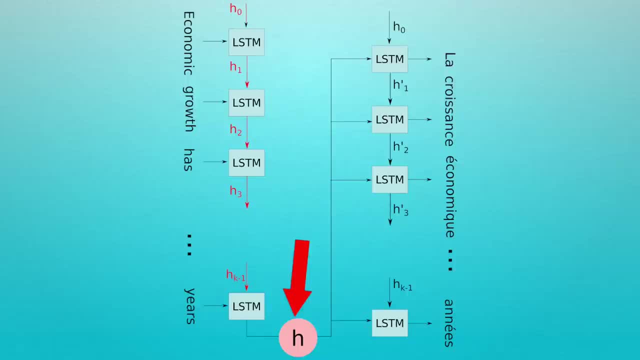 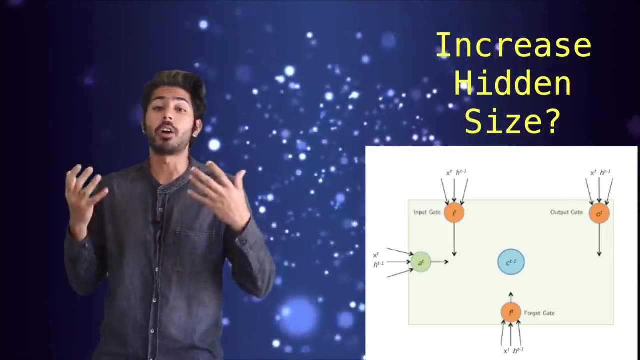 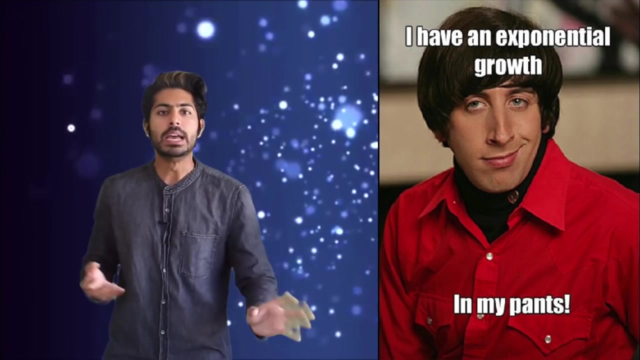 The more we try to force our sentence into this fixed dimensionality vector, the more lossy our neural net is forced to be. We could increase the hidden size of the LSTM- After all, they are supposed to remember long-term dependencies. But what happens is, as we increase the hidden size H of the LSTM, the training time increases. 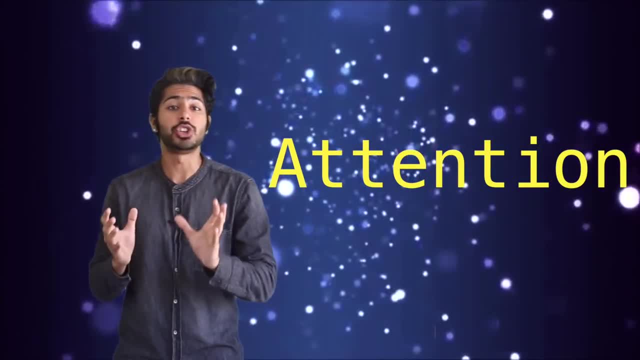 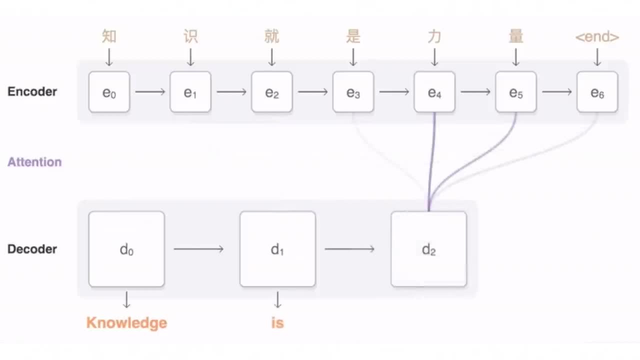 So to solve this, we're going to bring attention into the mix. If I was translating a long sentence, I'd probably glance back at the source sentence a couple times to make sure I was capturing all the details. I'd iteratively pay attention to the relevant parts of the source sentence. 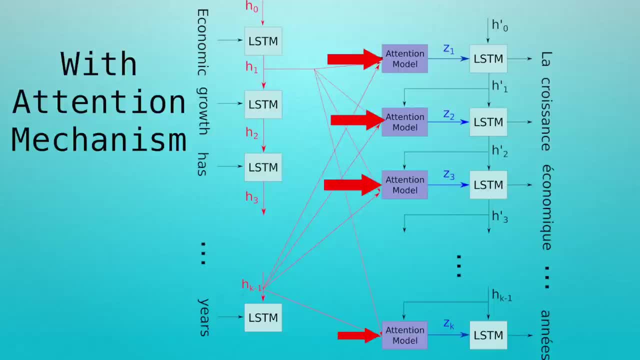 We can let neural nets do the same by letting them store and refer to previous outputs of the LSTM. This increases the storage of our model without changing the functionality of the LSTM. So the idea is, Once we have LSTM outputs, we can store and refer to the LSTM. 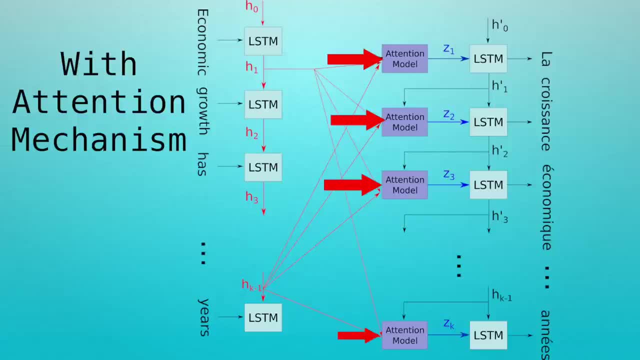 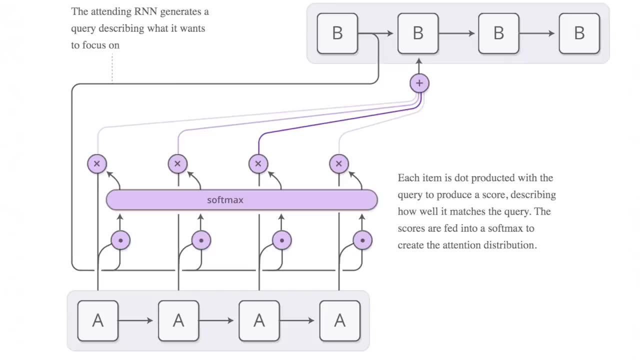 This increases the storage of our model. This increases the storage of our model So we can query each output asking how relevant they are to the current computation happening in the decoder. Each encoder output gets a relevancy score which we can convert to a probability score. 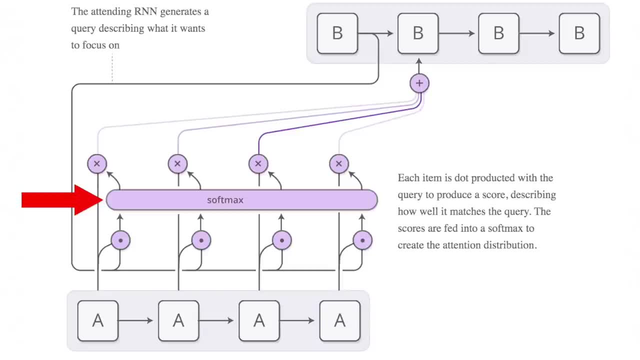 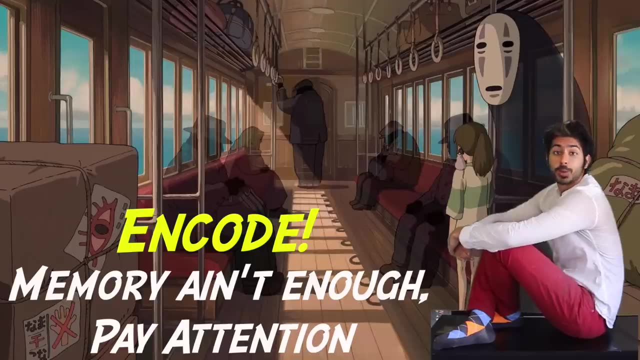 by applying a softmax activation to it. Then we extract a context vector which is a weighted summation to the encoder outputs, depending on how relevant they are. Memory ain't enough. Pay attention, I don't know what to do. What to do? 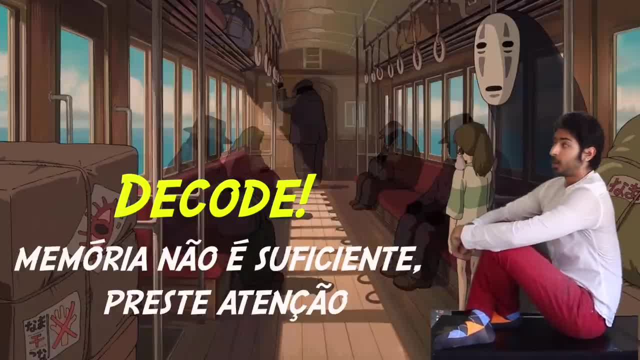 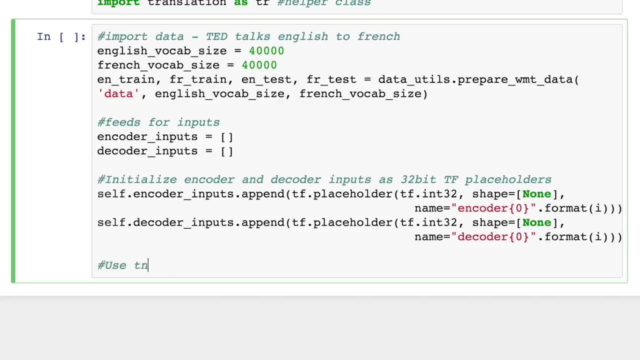 It's not enough. Pass it on, Memory isn't enough. Pay attention. We'll build our model using TensorFlow's built-in embedding attention sequence to sequence function, giving it our encoder and decoder inputs, as well as a few hyperparameters we define, like the number of layers. 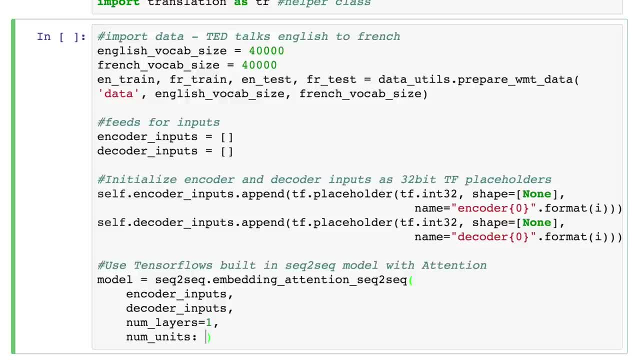 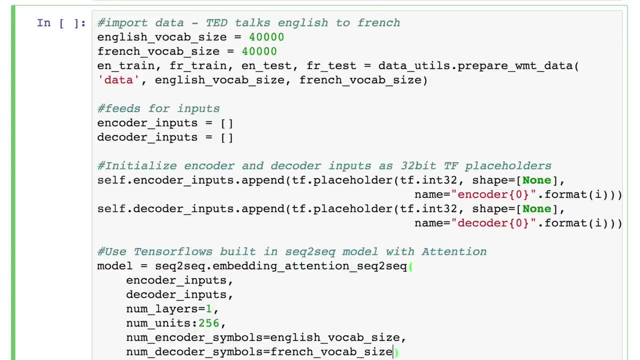 It builds a model that is just like the one we discussed. TensorFlow has several built-in models like this that we can drop into our code easily, So normally this alone would be fine and we could run this and the results would be decent, but they added another improvement to their model. 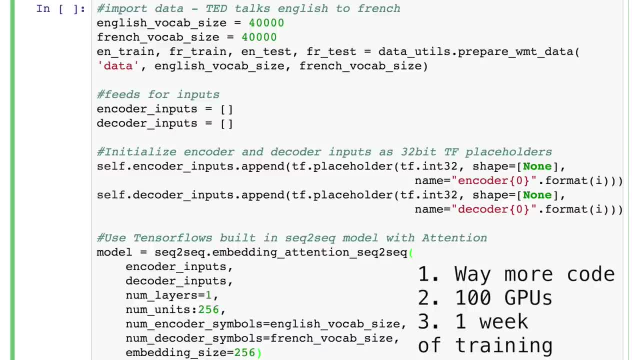 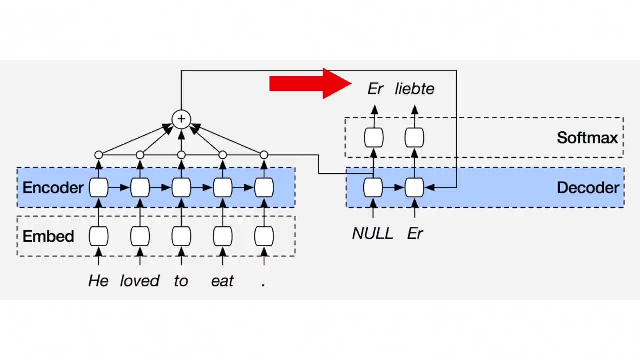 They added a model that requires more code, 100 GPUs and a week of training. Seriously, that's what it took. We won't implement it all programmatically, but let's dive into it conceptually. If the outputs don't have sufficient context, then they won't be able to give a good answer. 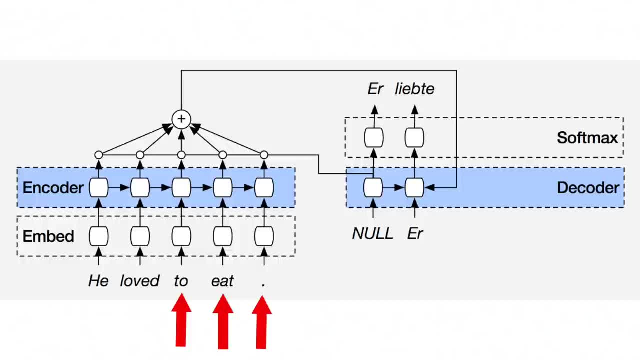 We need to include info about future words so that the encoder output is determined by words on the left and right. We humans would definitely use this kind of full context to determine the meaning of a word we see in a sentence. The way they did this is to use a binary. 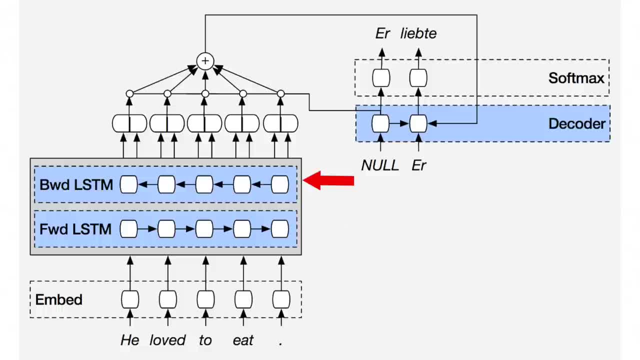 They used a bidirectional encoder, so it's two RNNs, one that goes forward over the sentence and the other goes backwards. So for each word it concatenates the vector outputs, which produces a vector with context from both sides, And they added a lot of layers to their model. 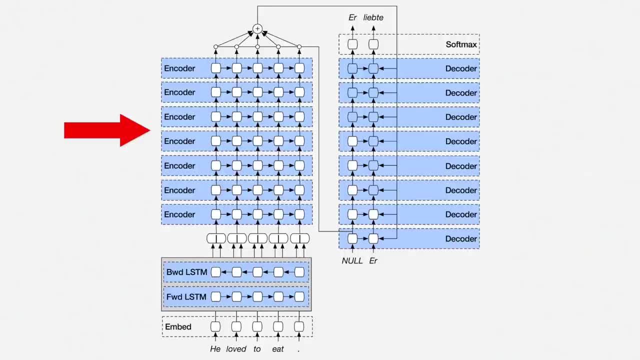 The encoder has one bidirectional RNN layer, then seven unidirectional RNN layers. The decoder has eight unidirectional RNN layers. The more layers, the longer the training time. so that's why we used a single bidirectional layer. If it's unidirectional, the whole layer would have to finish before later dependencies could.